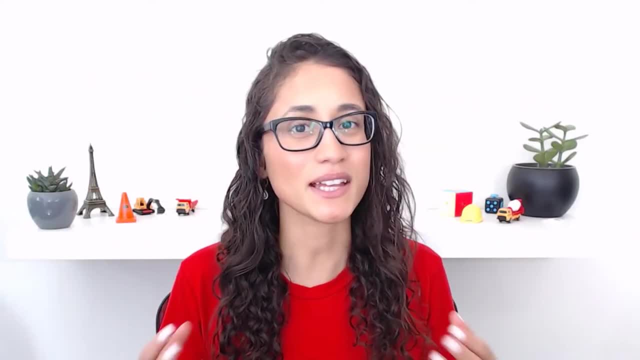 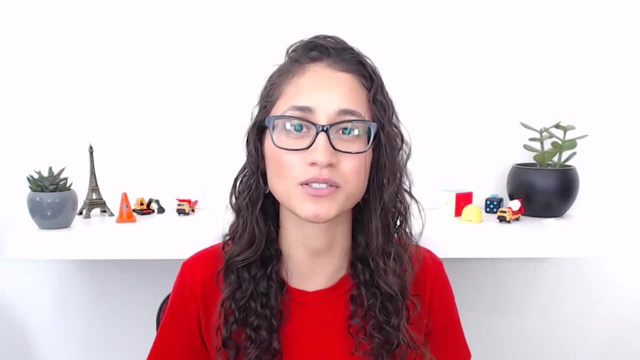 Bonjour génie ingénieurs. Welcome to my problem a day series. In this video we're going to do the last part of the previous problem. We're going to calculate how long would it take for 50% consolidation. These type of problems are important if you're taking FE, civil or 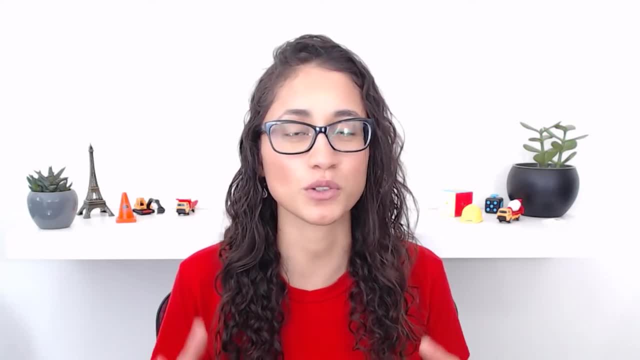 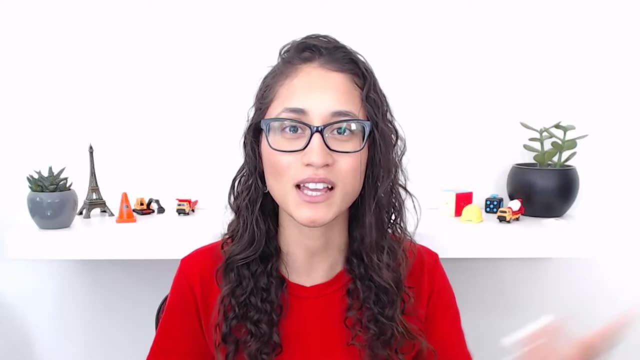 soil mechanics class. Now, if you're here for the first time and you just want to learn about engineering or just how to engineer a better life, don't forget to subscribe and make sure you hit the bell so you don't miss out on future videos. Now let's get started. 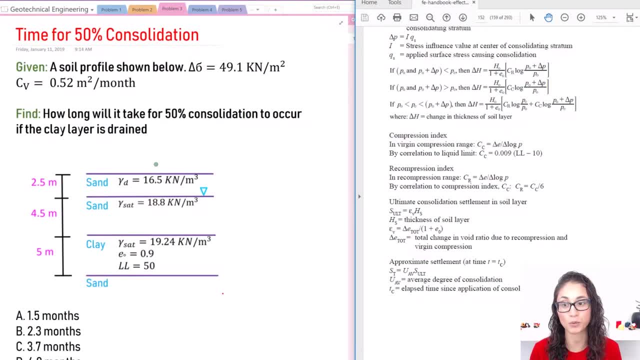 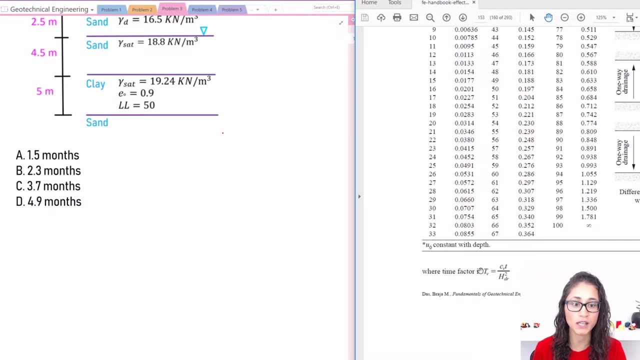 Okay, guys. so this is the last part of the previous problem that we did. Now here we need to calculate the how long it would take for 50% consolidation to occur if the clay layer is drained. Okay, so we're pretty much looking for the time. So, if you go to page 153, 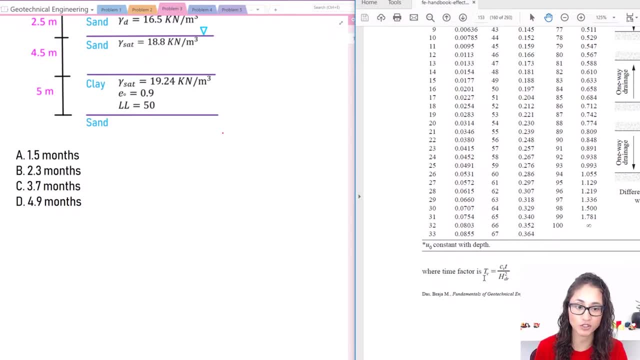 as we mentioned in the previous video. here we have the time factor and from TV we can calculate T, because we were given the degree of consolidation. We can find TV from there, our height drainage we already have and CV and all we need to do is calculate the time and that's. 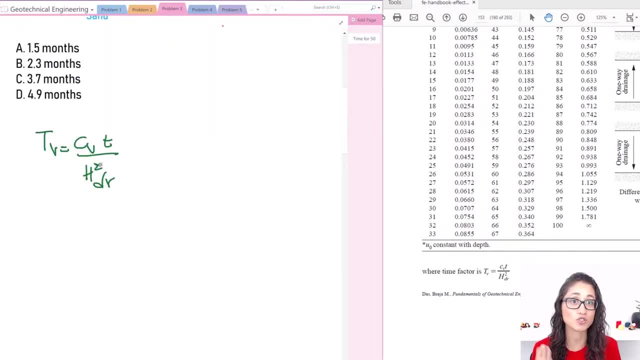 what we're looking for. So let me write the equation down. Okay, guys, so know that we're trying to look for the time for 50% consolidation and we're not really trying to look for a time factor. in fact, when you are giving the degree of consolidation, you can easily determine the. 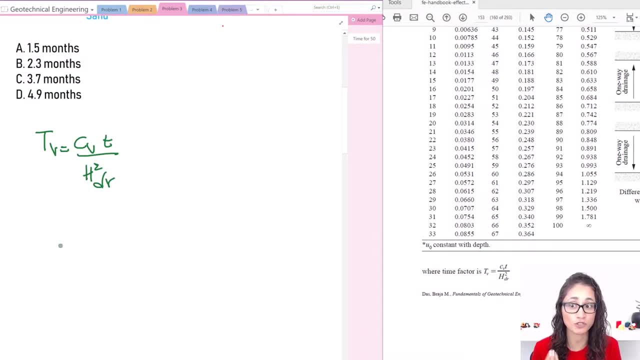 time factor. So let's rearrange this equation and solve for T. So I have: T is equal to TV, my height drainage squared divided by 7.. So we said, to calculate TV we're going to use the degree of consolidation, which is 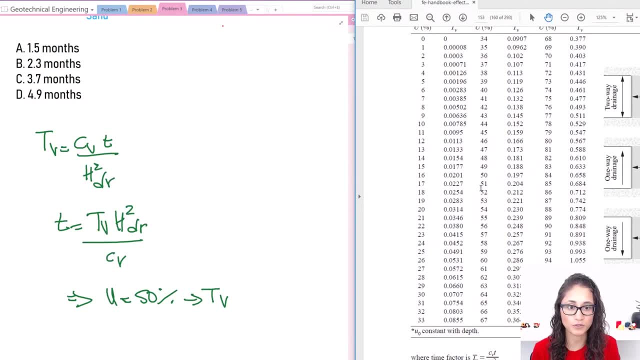 50%. If you go to the tables on page 153, you'll see here that your 50% consolidation gives us a time factor of 0.197.. So let's write that down. So I have 0.197.. So if I plug in here all my numbers, I can easily solve for our time. 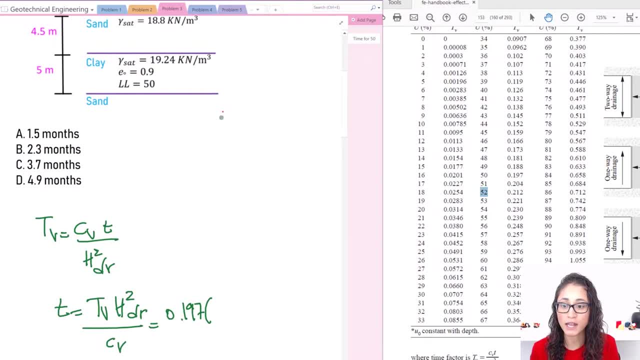 So our high drainage, as we mentioned in the previous video, it's going to be 2.5, because I have clay that is between sand, two sand, two layers of sand, And so, which means I'm going to have two-way drainage.